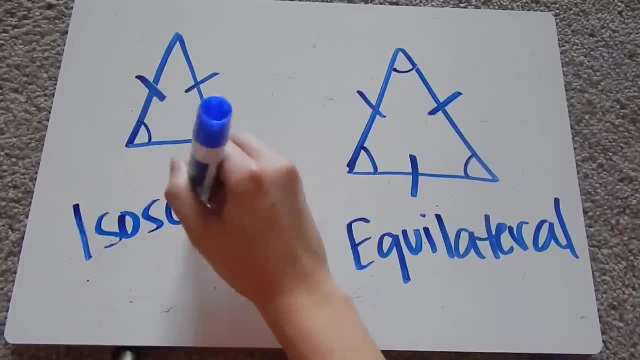 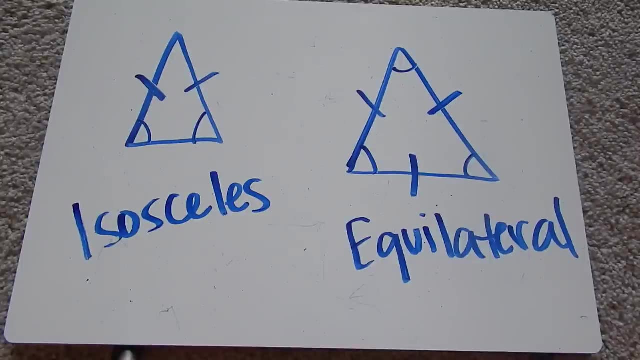 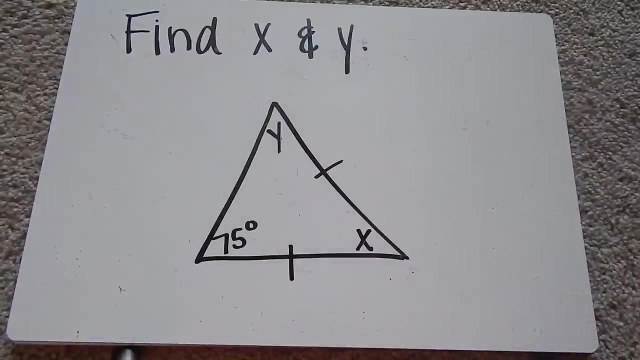 And this is the isosceles triangle theorem. Again, if you have two or three congruent sides, the angles opposite of the sides will also be equal. So let's move on to some examples. The first one says: find x and y. 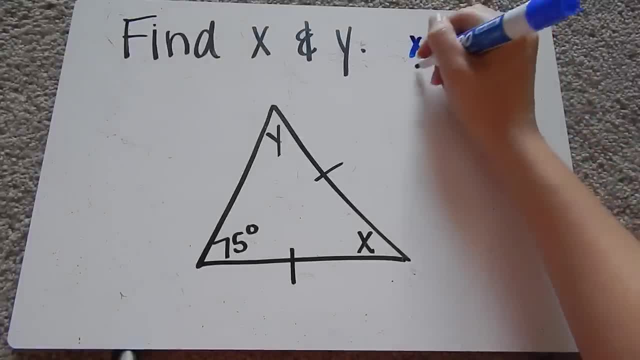 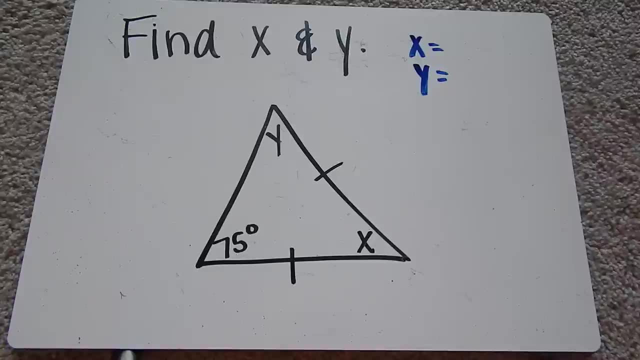 So we want to find x And we want to find y. Well, if you notice, we have a triangle with two equal sides. This is an isosceles triangle. So when we have two congruent sides, the angles opposite of the sides. 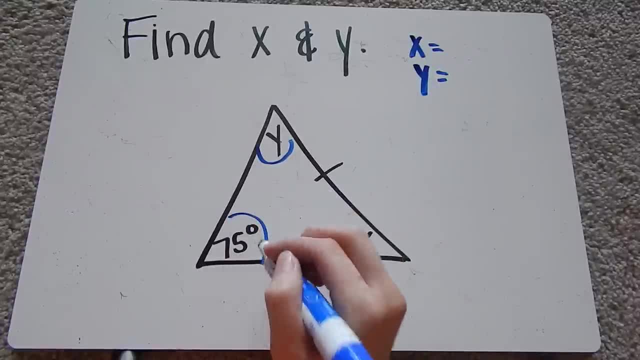 so this angle here and this angle here will be congruent. Well, I already know: one of the sides or one of the angles is 75. The other angle must be 75. So y is equal to 75. That was easy enough. 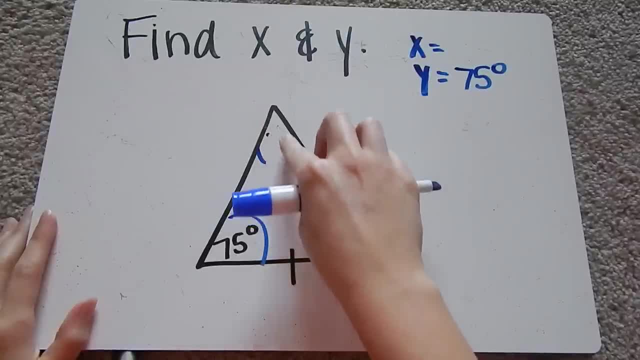 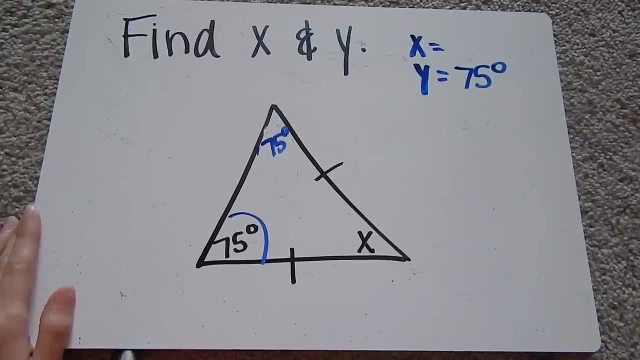 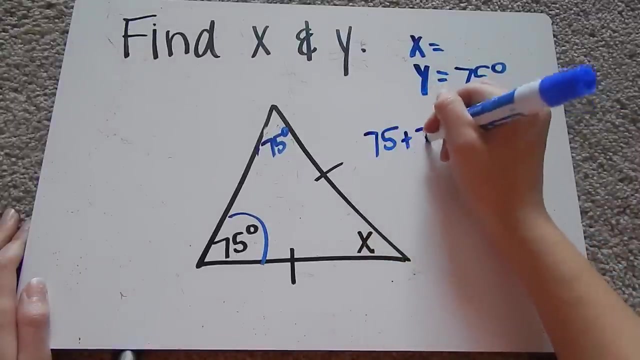 Now let me go ahead and erase this And put the actual measure. This is now 75 degrees. So now we can easily figure out x, Because all angles of a triangle add up to 180.. So x is going to be 75 plus 75 plus x equals 75.. 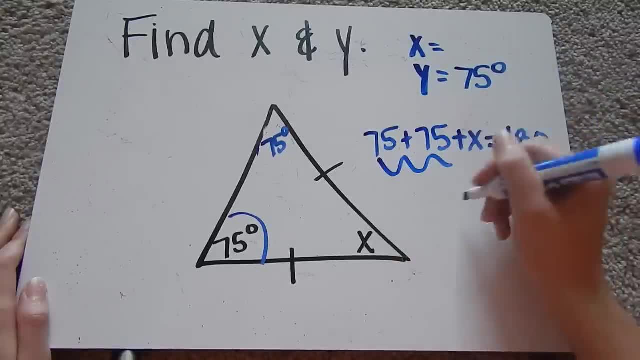 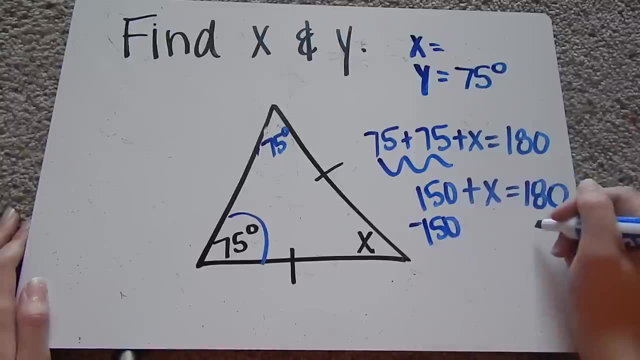 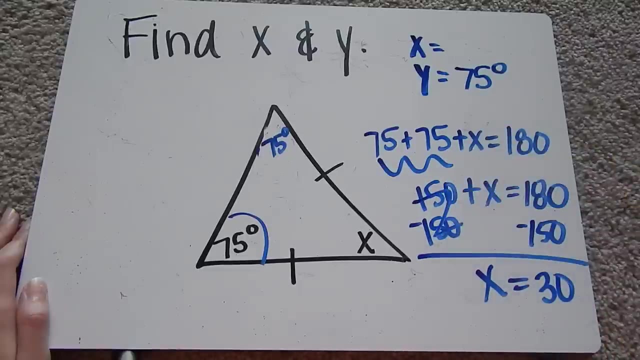 Plus x equals 180.. Combine like terms: 150 plus x equals 180.. Subtract 150 from both sides, x equals 30. These will zero out, So x is 30 degrees. So those are our answers to this example problem. 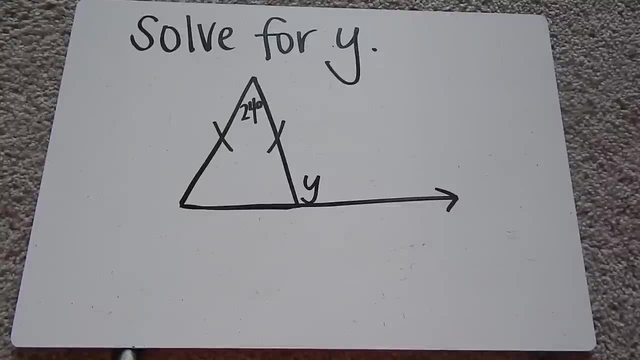 Moving on to the next problem. This problem says: solve for y. Again, I have two congruent sides, which means these bottom angles are going to be congruent. If I can figure out these bottom angles, then I can figure out this exterior angle. 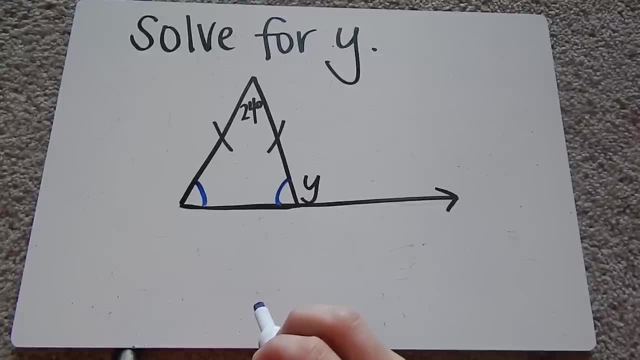 by using our exterior angle theorem. So, because I have two congruent angles, I'm just going to name this. I'm going to call them x. They're both equal to x. All three angles of a triangle add up to 180. 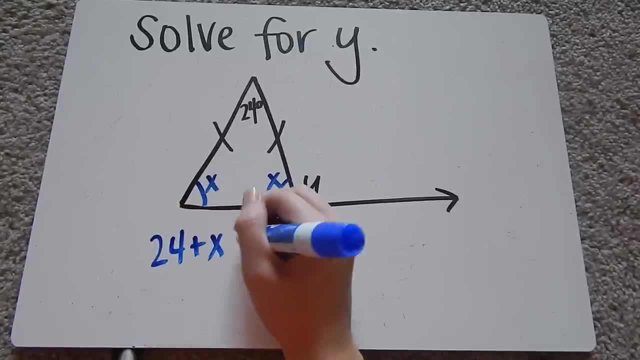 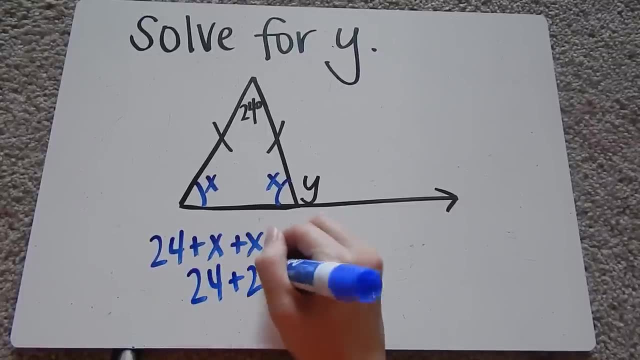 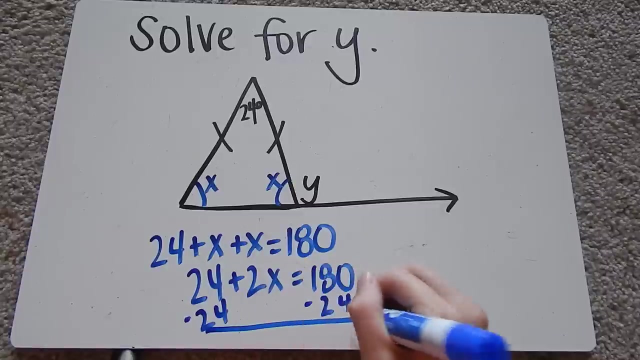 So we do: 24 plus x plus x equals 180.. So 24 plus 2x equals 180.. Subtract 24 from both sides, The 24's will zero out. We get 2x equals 180.. The 24's will zero out. 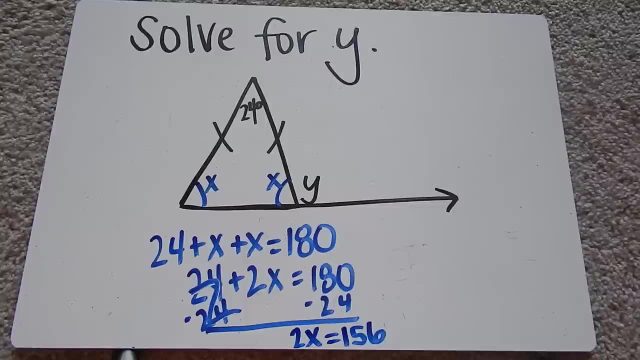 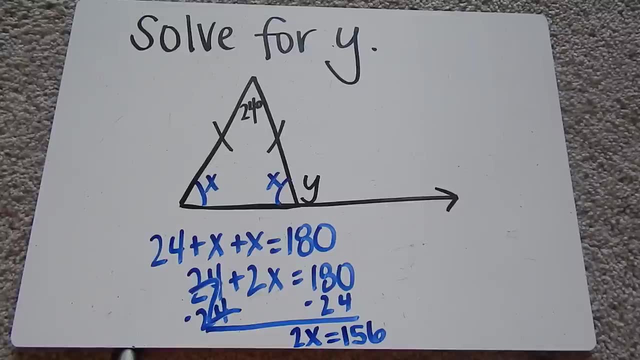 We get: 2x equals 156. And then we're going to go ahead and divide both sides by 2. So 156 divided by 2. I'll just bring that over here: x equals 78. So both of these angle measures equal 78.. 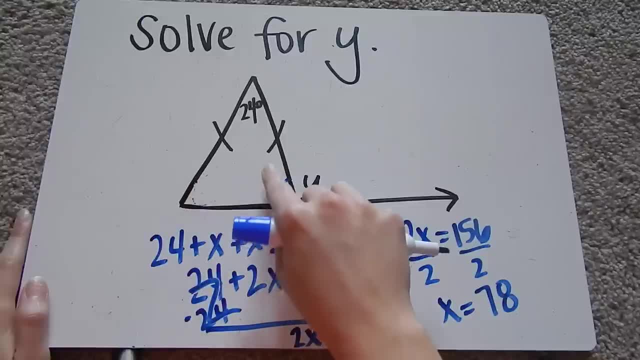 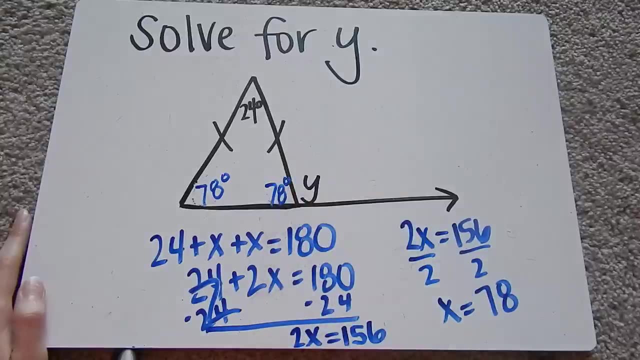 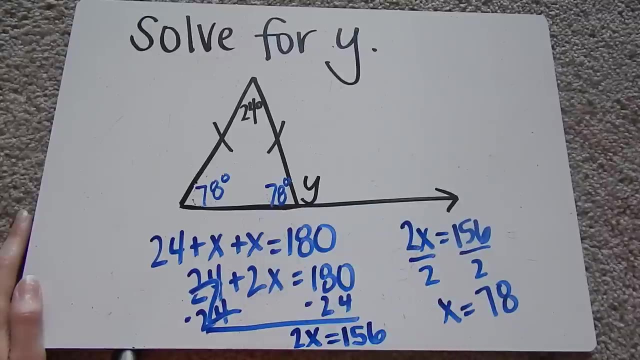 I'm going to write that in. Once we have these angles, we can find y two different ways. One is: you can recognize this is a line. Straight lines form together add up to 180 degrees, So you can just use this angle to find y. 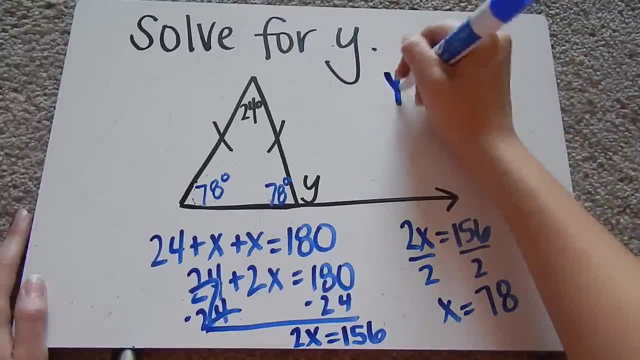 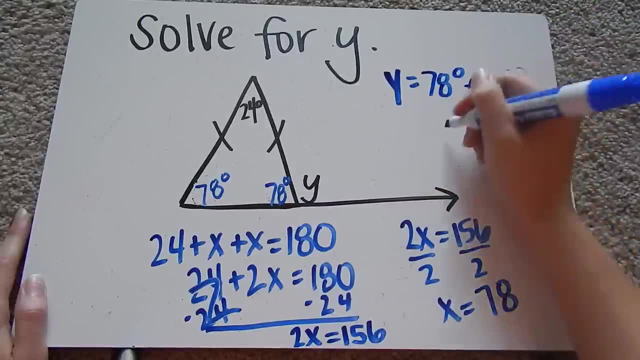 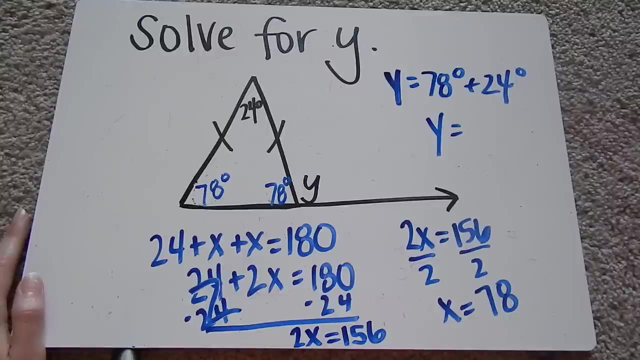 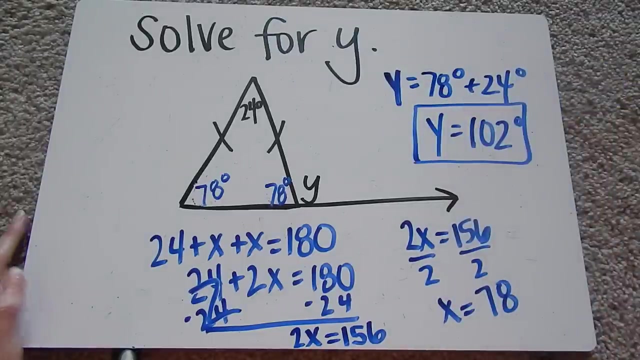 Or y. the exterior angle is equal to the sum of the remote interior angles: 78 degrees plus 24 degrees. So either way would get you your answer. 78 plus 24 is going to be 102 degrees. So that is my answer. 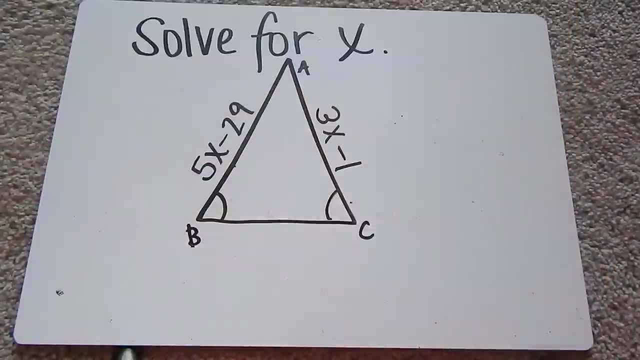 That is y. And our last example. It says: solve for x. So in this problem we're actually going to work backwards. We know that these angles are equal. That means that the opposite sides of the angles are equal. It works both ways. 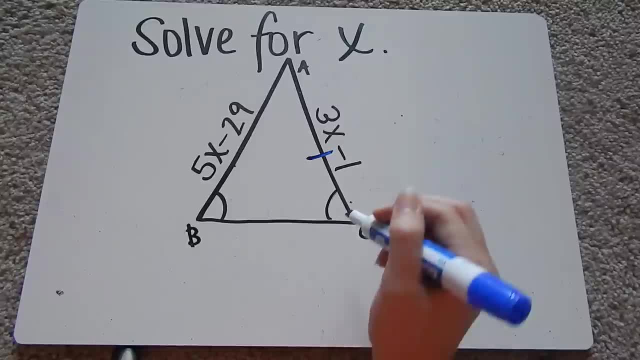 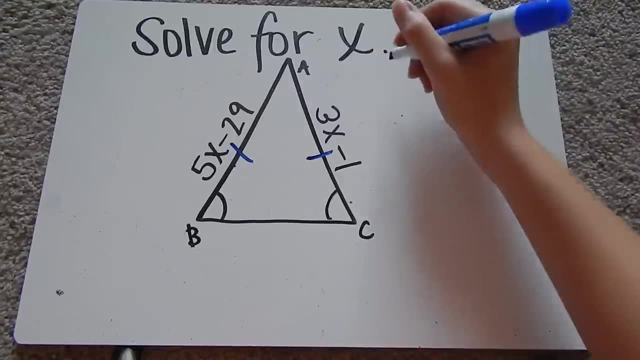 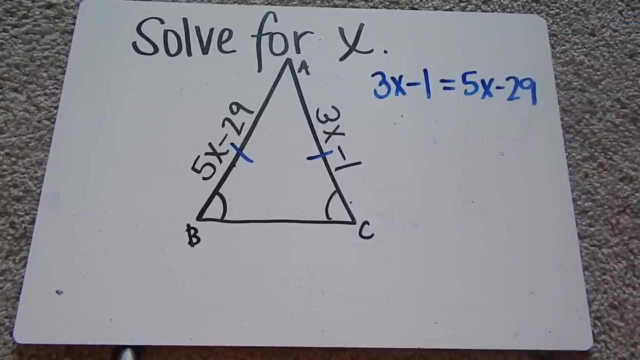 So this angle here means that side, This angle here means that side- are equal. Since these two sides are equal, we can set them equal to each other and solve: 3x minus 1 equals 5x minus 29.. Okay then, I'm going to move all the x's to one side.